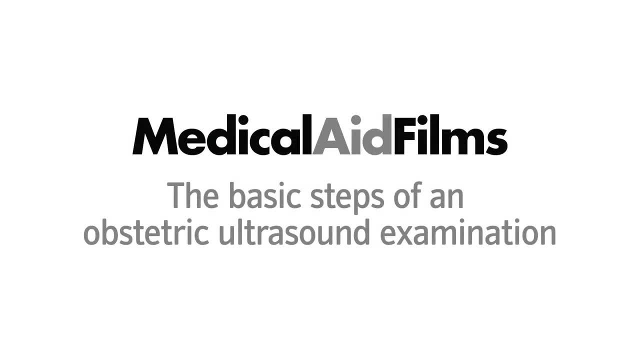 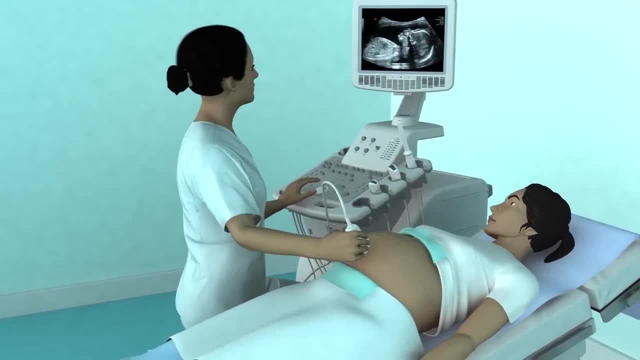 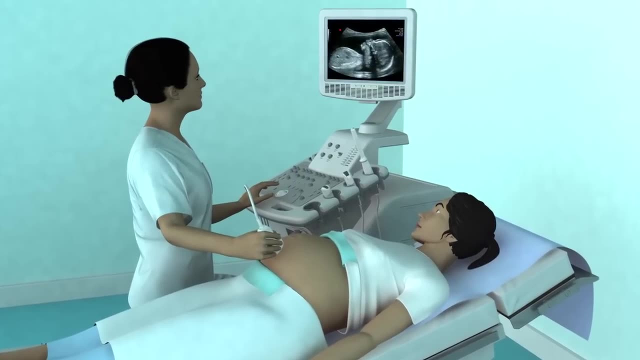 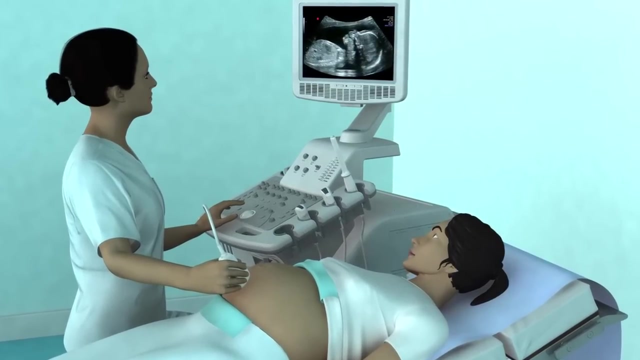 Ultrasound allows accurate estimation of gestational age, determination of fetal viability and presentation position of the placenta, measurement of amniotic fluid, estimation of fetal weight and identification of multiple pregnancies. It can also be used to detect some fetal abnormalities. 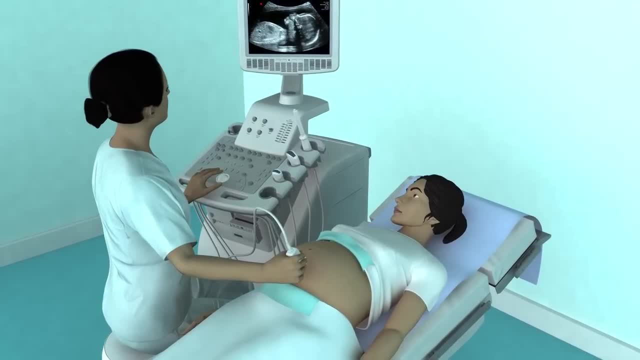 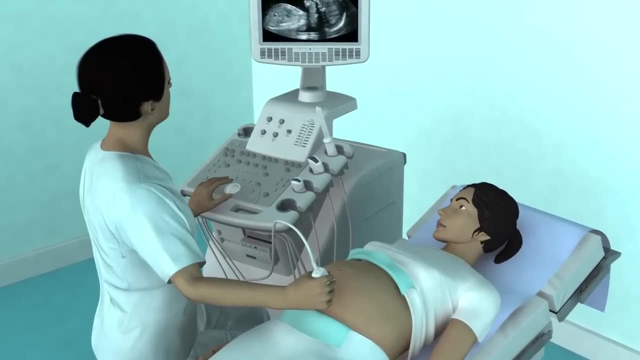 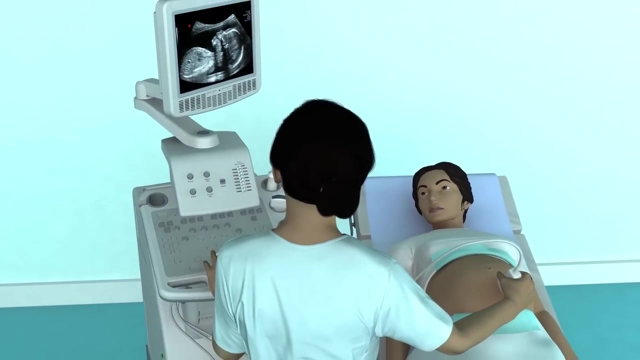 This film will show you how to prepare for scanning, how to examine and measure the foetus using both the standardised six-step approach and part of ISOOG's twenty planes and two sweeps approach, and, finally, how to provide aftercare for the woman. The examples used: 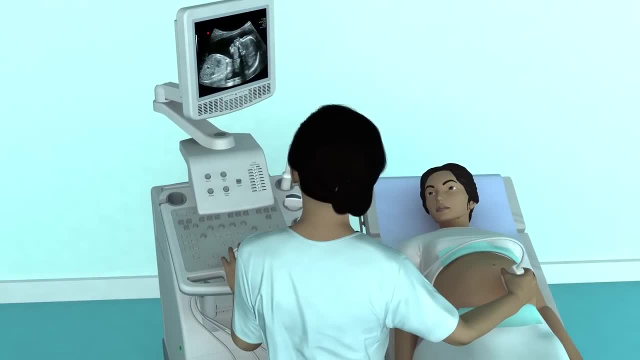 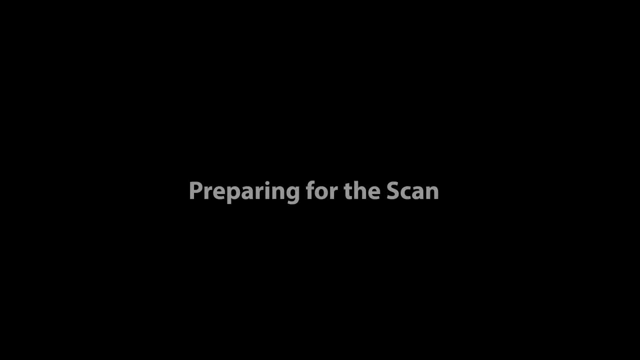 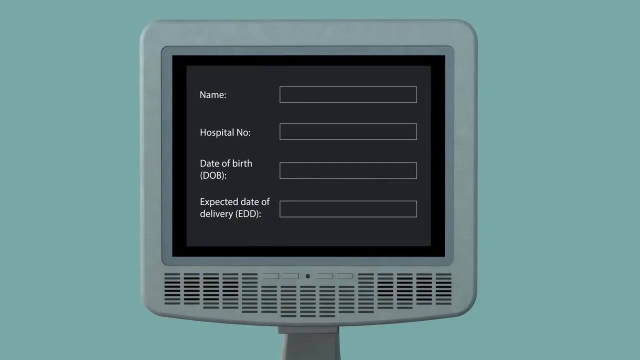 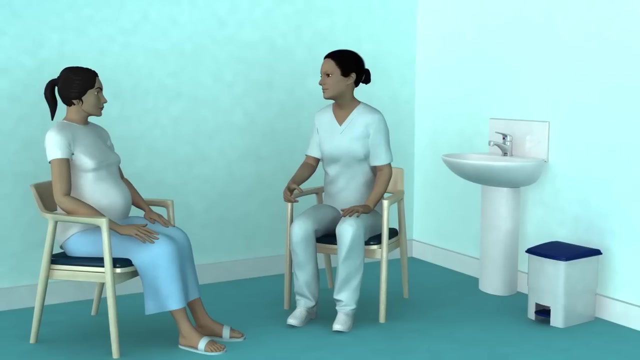 will incorporate pregnancies of different gestations to best illustrate the specific steps of the scanning procedure. Before starting the ultrasound scan, enter the woman's details and confirm them with her. Explain the process and the indication for the scan. Make sure she is ready to proceed. 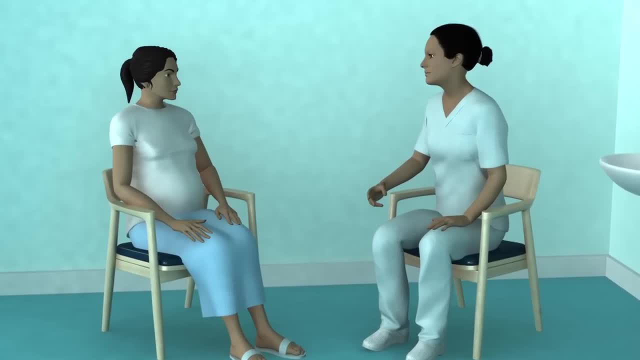 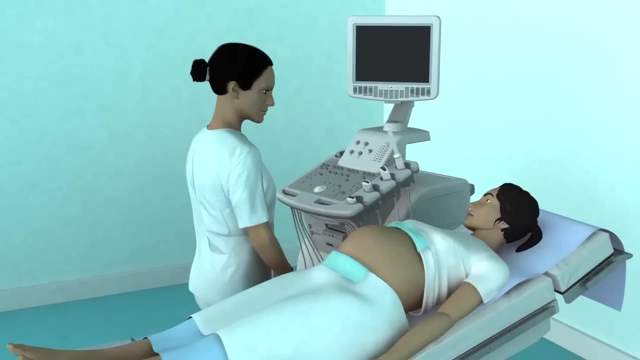 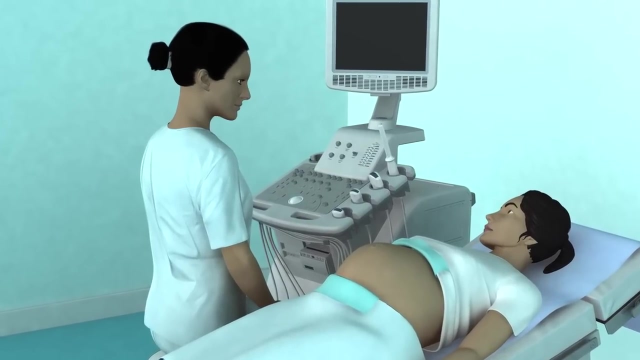 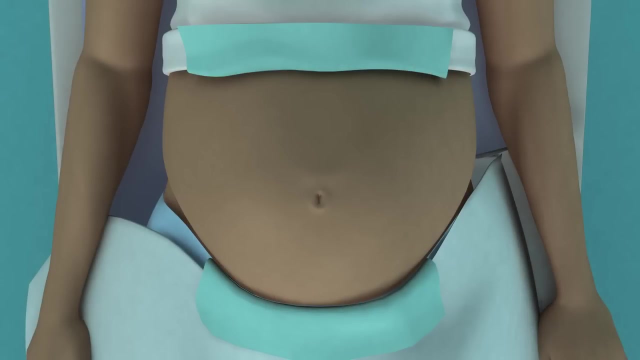 and answer any questions she may have. Although there can be exceptions, the scan is usually performed with the woman lying to the right of you and facing you. Adjust the height of the couch and stool to allow you to work in a comfortable position. The woman should be properly covered and her clothing protected from the ultrasound gel. 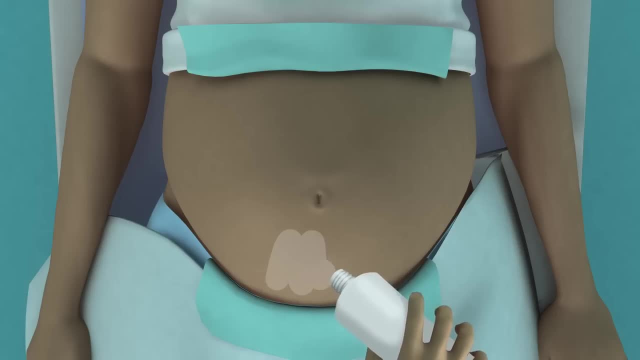 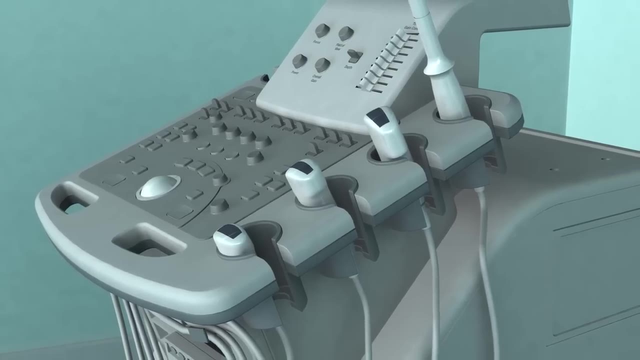 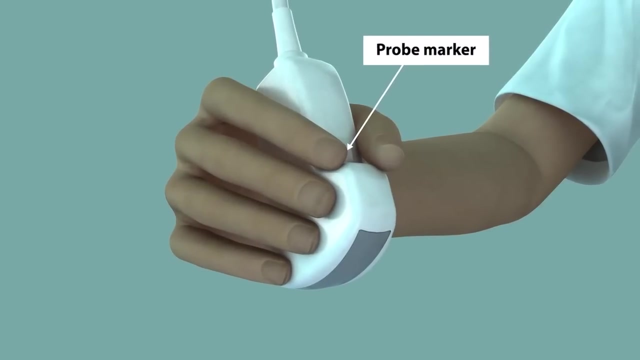 Now apply the gel over her lower abdomen. Select the probe and preset which are most suitable for the gestational age and body mass index, or BMI, of the woman. Hold the probe and press the BMI button. Hold the probe with your right hand and operate the machine controls with your left. 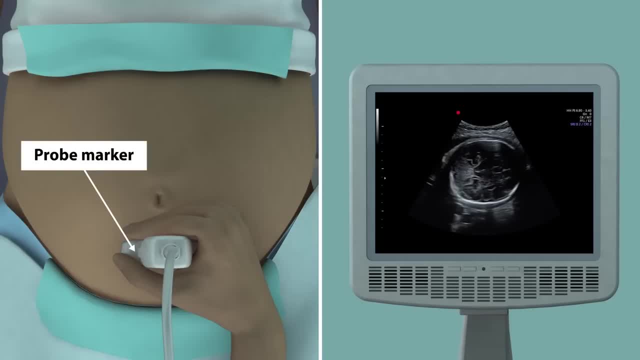 Placing the probe in a transverse position on the lower abdomen. use its marker as a reference to make sure that the right side of the mother is displayed on the left side of the screen. You can check this by pressing your finger beside the probe in the abdomen. 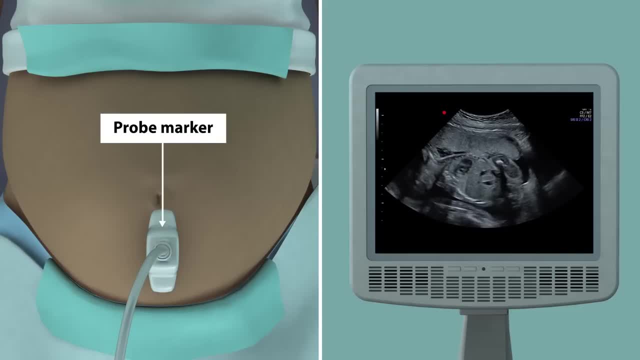 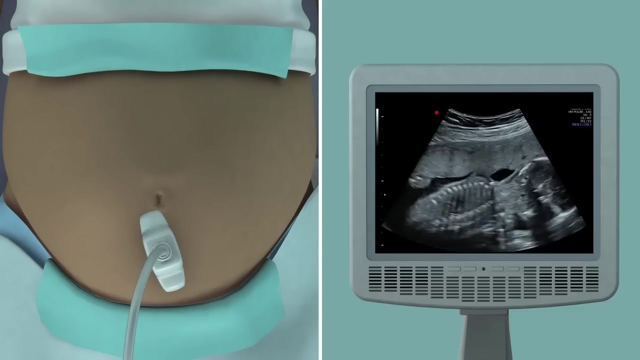 Placing the probe in a longitudinal position and using its marker as a reference, you can see that the uterine fundus should be displayed on the left side of the screen and the maternal bladder on the right. To keep the image orientation correct, rotate the probe in a clockwise direction when changing. 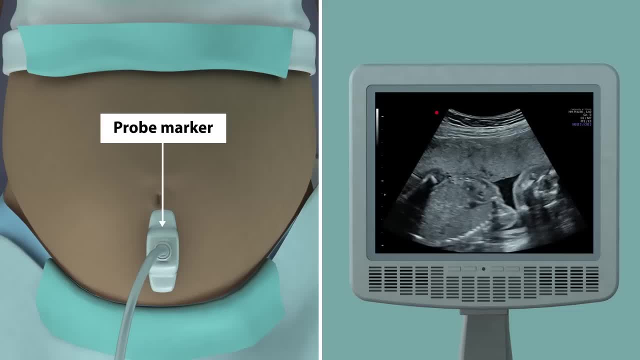 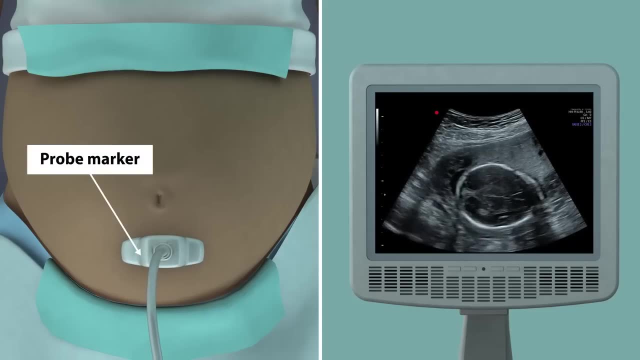 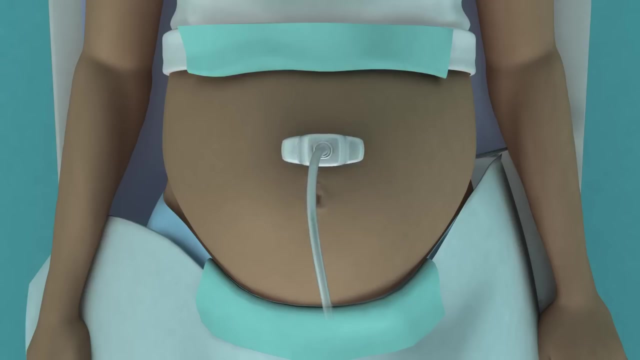 from a transverse plane to a longitudinal plane, and anticlockwise. when changing from longitudinal to transverse, Always keep the orientation of the probe consistent and don't rotate it more than 100 degrees. The probe can only be moved in four ways: by sliding, rotating, dipping or angling. 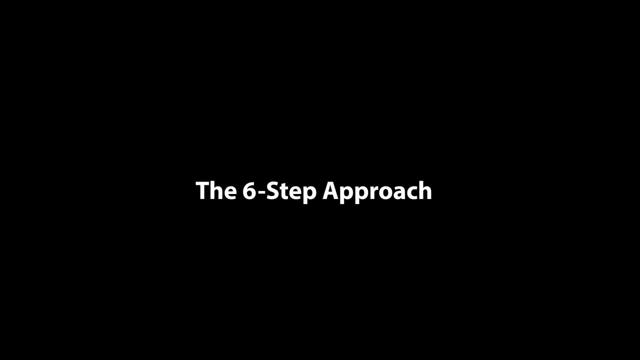 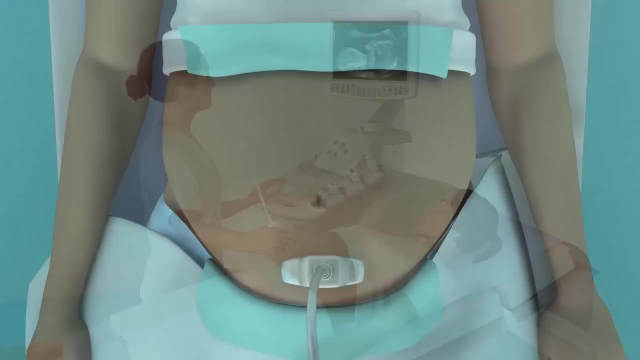 Isuog recommends using the six-step approach for the performance of a basic, second or third trimester obstetric ultrasound examination. The first step is to place the probe in a transverse position in the centre of the lower abdomen, just above the symphysis Angle. the probe forwards and backwards to identify the 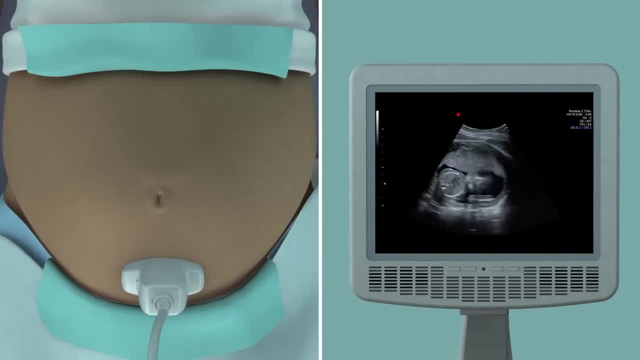 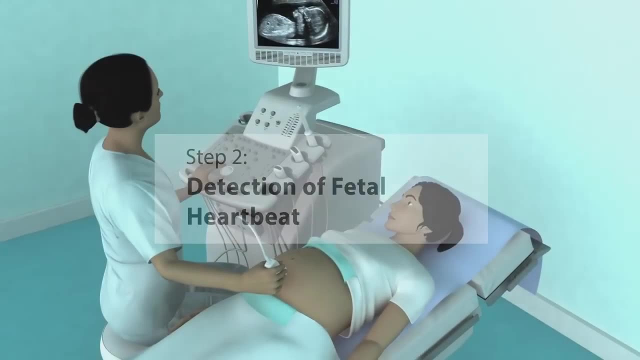 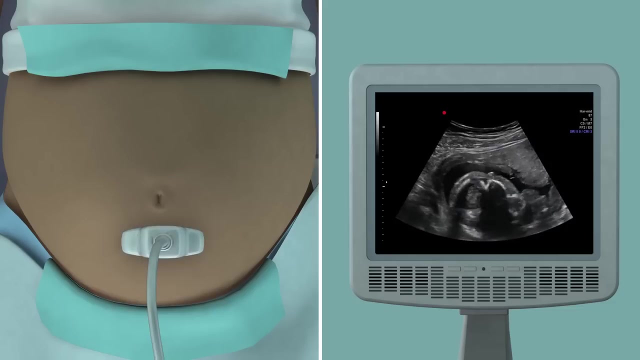 presenting foetal part. This foetus is cephalic, Maintaining a transverse orientation. slide the probe up towards the maternal umbilicus to identify the foetal heart and heartbeat. If the foetal heart is not seen in this sweep, slide the probe to the maternal right and. 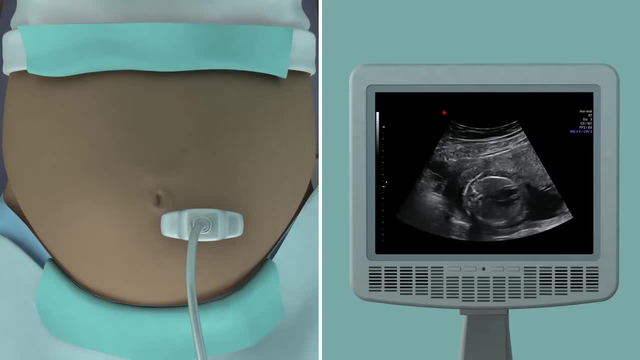 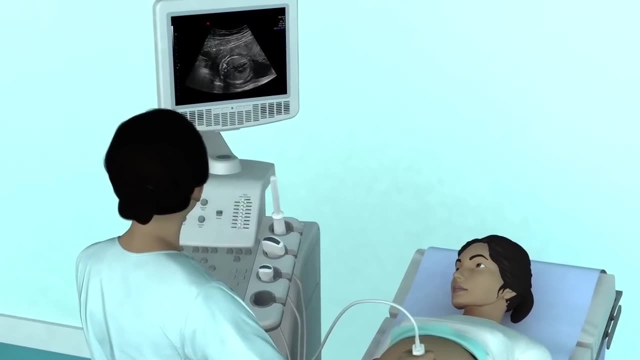 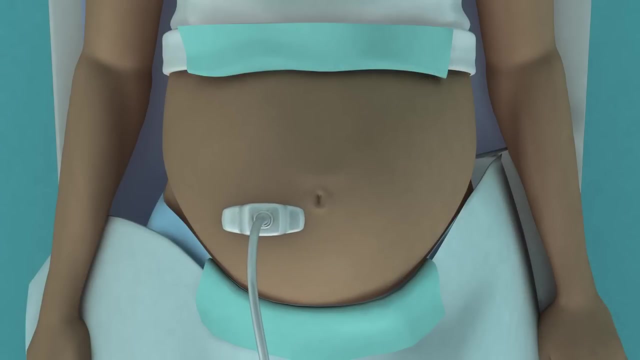 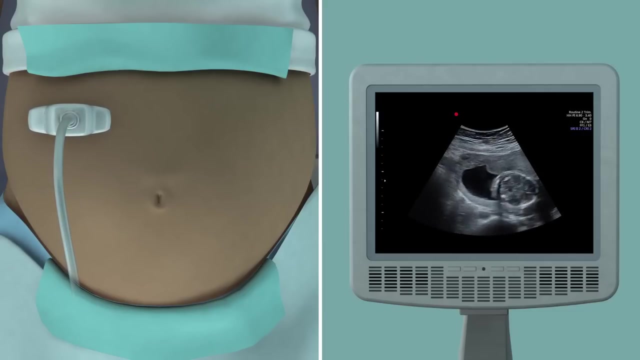 then left to locate it and confirm that the heart is beating. Let the woman view the screen Maintaining the transverse orientation. slide the probe up the right side of the uterus, from the symphysis to the fundus. Repeat this movement in the centre of the uterus and also in the left side of the uterus. 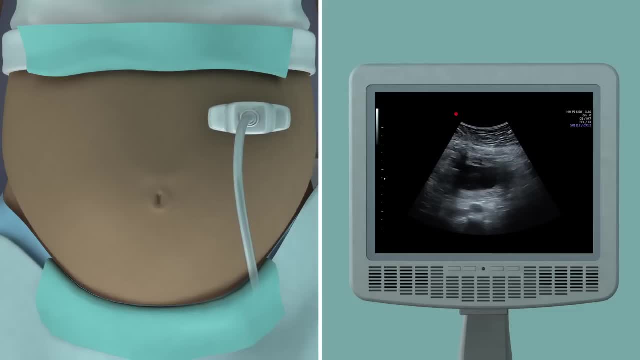 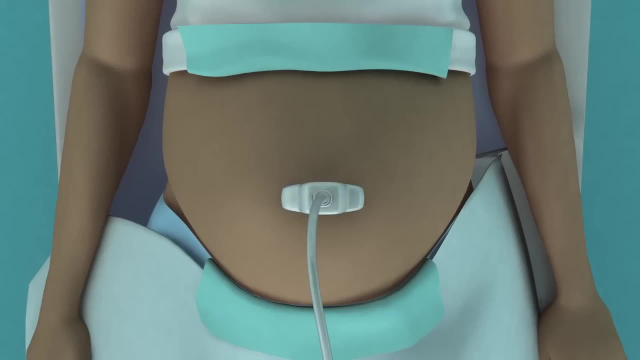 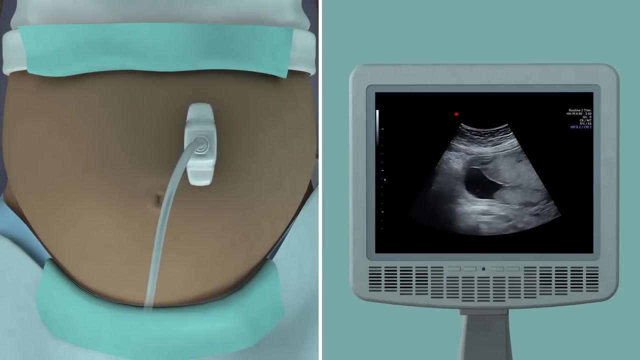 The size of the uterus will determine whether two or three transverse sweeps are required To complete this step. make sure that the uterus is in the centre of the uterus, rotate the probe to a longitudinal position and survey the whole uterus by sliding the probe from the right side to the left, above and below the umbilicus. 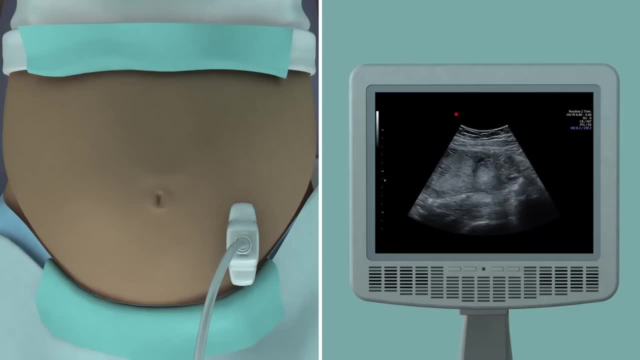 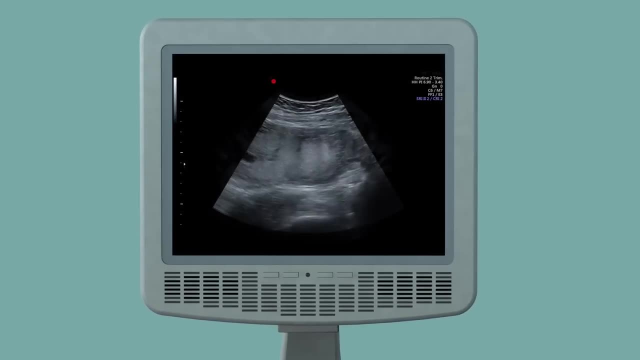 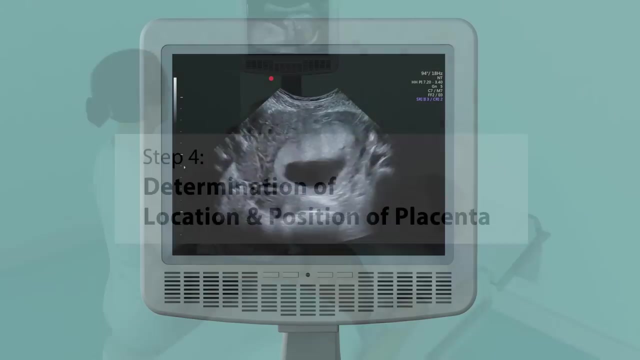 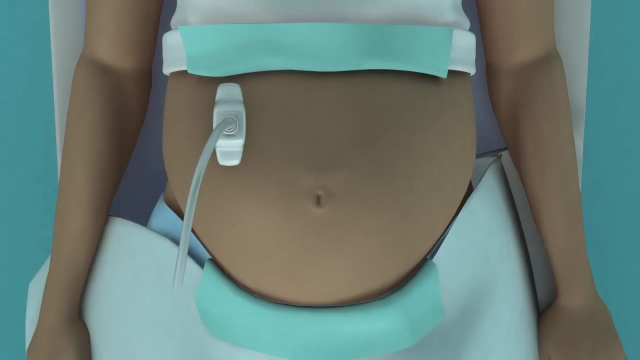 Keep the probe perpendicular to the floor. as you slide it, The screen here shows a singleton and here you can see twins Maintaining a longitudinal orientation, starting at the right fundus. slide the probe down towards the symphysis, keeping it perpendicular to the floor. 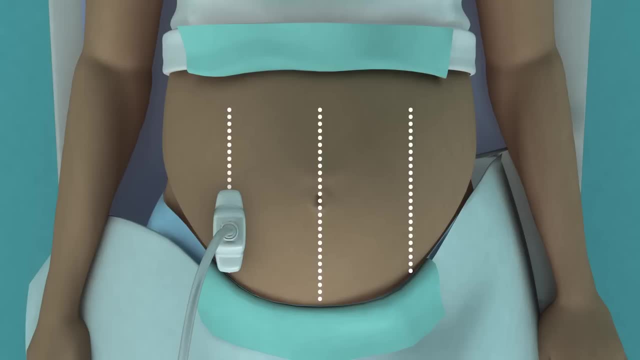 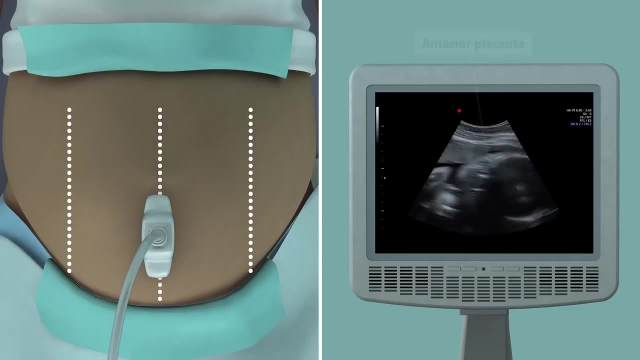 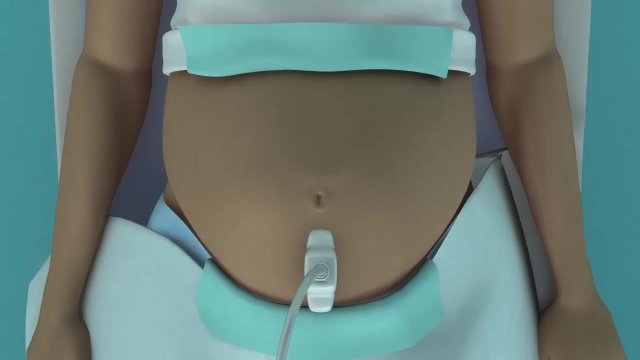 Slide along the three tracks indicated to identify the location of the placenta. Here you can see first anterior, then posterior and here a low-lying placenta. Slide the probe into the midline and, using small movements, locate the leading edge of. 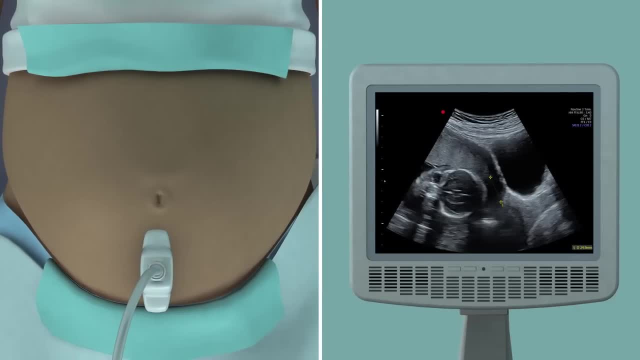 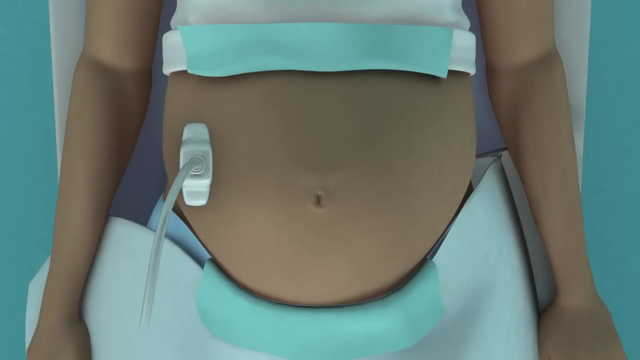 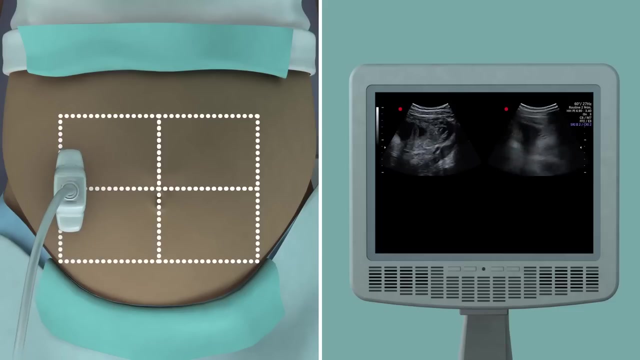 the placenta in relation to the internal os. Here you can see a low-lying anterior placenta. Mentally divide the maternal abdomen and uterus into four quadrants. Keeping the probe in longitudinal orientation and perpendicular to the floor, slide it from the lower right quadrant through the other three quadrants. 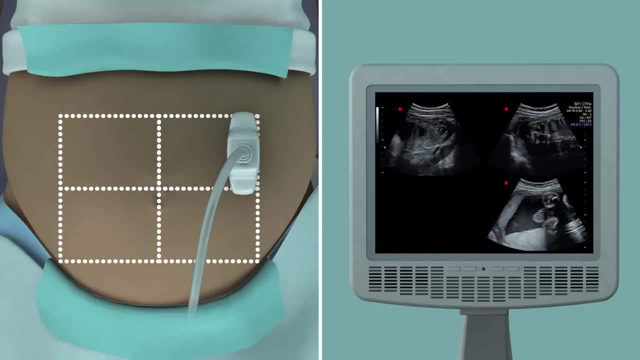 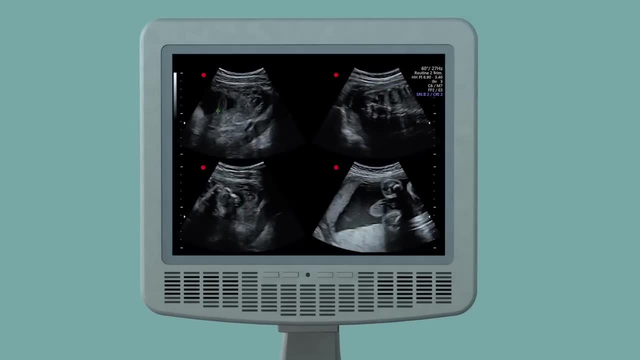 Identify the deepest vertical pocket of amniotic fluid in each that does not contain any foetal parts or umbilical cord, and measure by placing the callipers at 90 degrees to the horizontal. The amniotic fluid index, or AFI, is the sum of these four measurements. 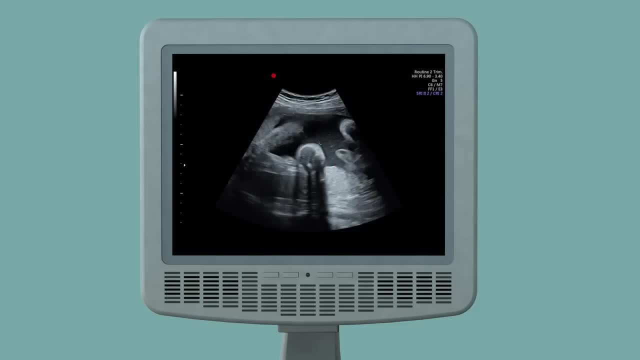 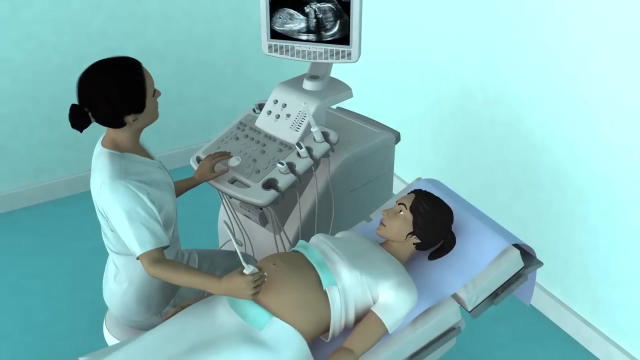 The deepest vertical pocket, or DVP, is the largest measurement of the four. Beware here of reverberation artefacts that could make you underestimate one or more of these. Thank you for your attention. these measurements, To take the biometric measurements, apply the first sweep and planes 4, 5, 7 and 11. 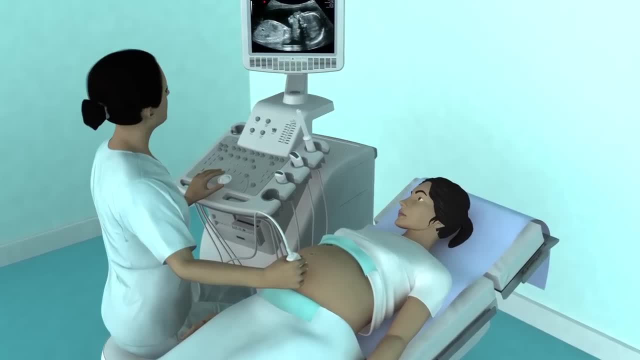 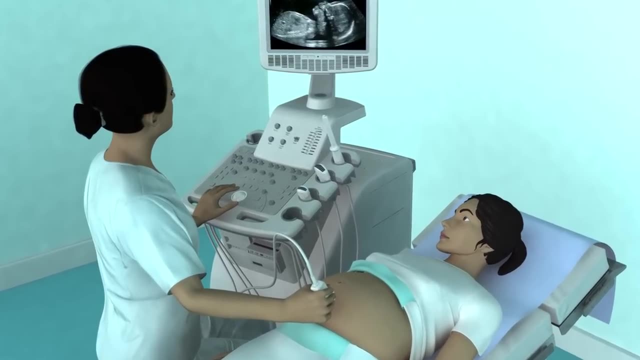 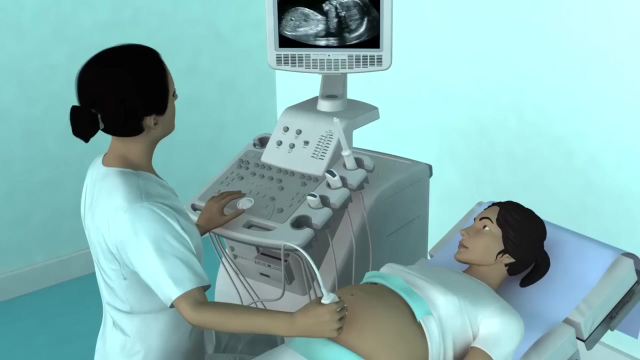 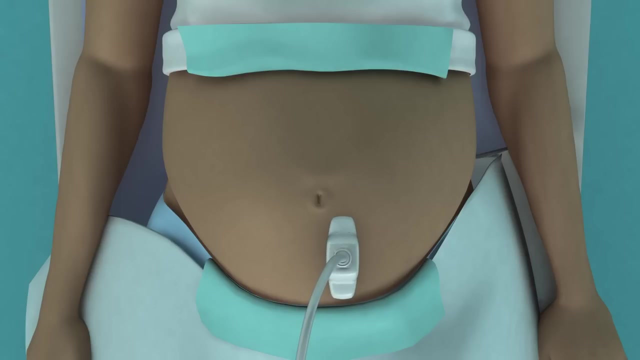 of ISSU-OG's standardised 20 planes and 2 sweeps approach. It is good practice to take each measurement at least three times to make sure your technique is consistent. Restore each measured image on the machine. Perform the first sweep by rotating the probe to obtain a longitudinal section of the foetus. 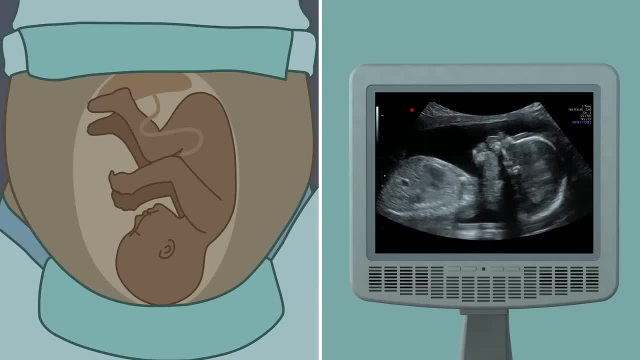 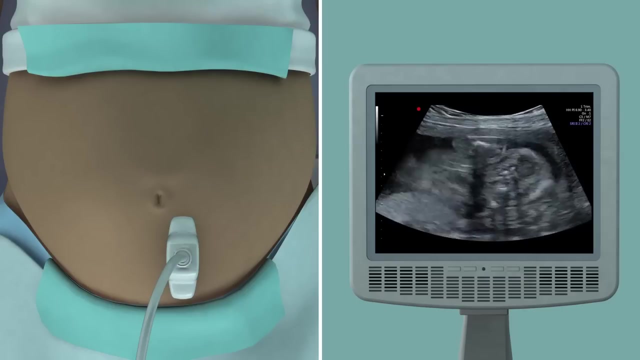 Identify the positions of the foetal head and long axis of its body. The first measurements to take are the biparietal diameter, or BPD, and head circumference, or HC, From the longitudinal axis of the foetus. rotate the probe by 90 degrees at the level of the foetal head. 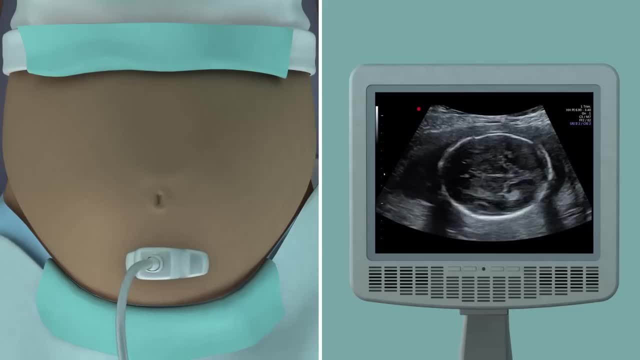 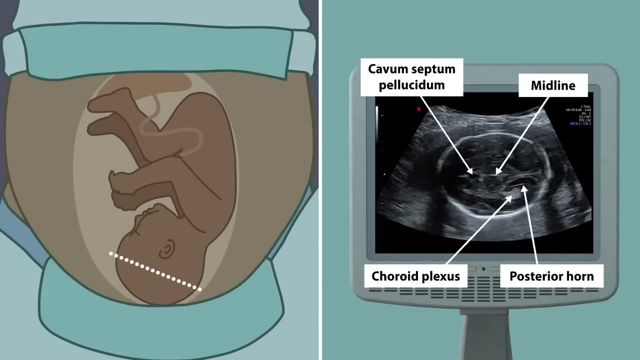 Angle, slide, rotate and then dip the probe to obtain the correct head shape and intracranial landmarks which indicate the transventricular plane known as plane 4.. Take the biparietal diameter measurement at the widest point across the skull. Depending on local charts, the BPD may be measured. 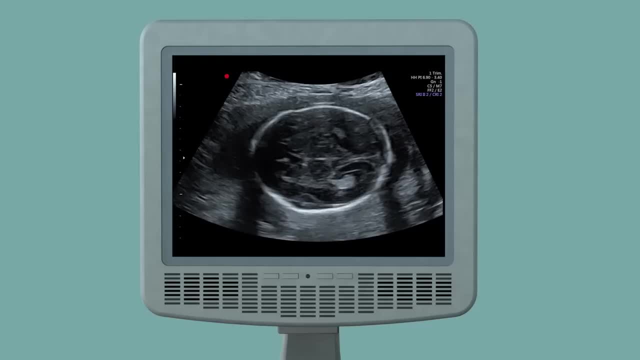 outer to outer or outer to inner? To obtain an outer to outer BPD measurement, place the calipers on the outer edge of both upper and lower parietal bones. To obtain an outer to inner BPD measurement, place the lower caliper on the inner border. 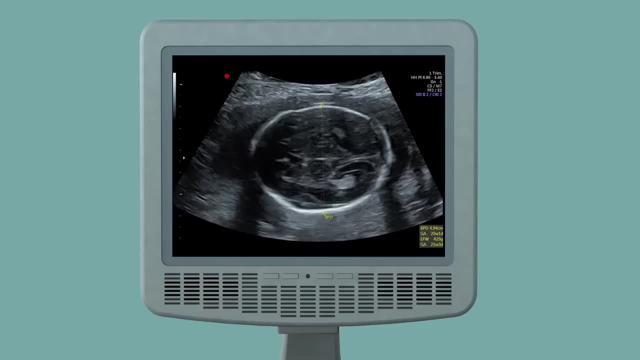 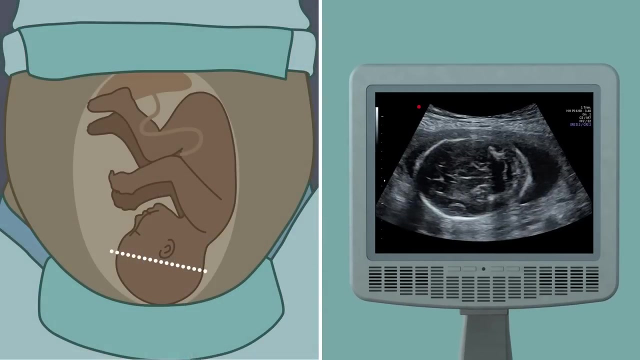 of the lower parietal bone. Next, measure the head circumference by placing the ellipse caliper on the outer edge of the skull. Then rotate from the transventricular plane to the transcerebellar plane or plane 6, by keeping the cavum septum pellucidum in view and rotating the probe towards the foetal. 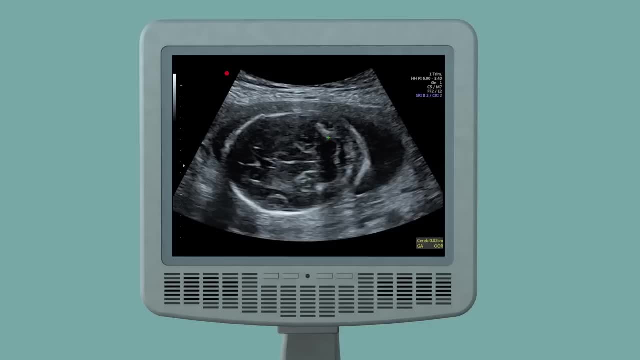 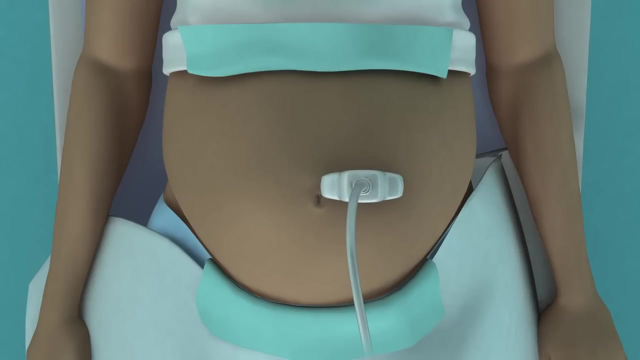 neck. Measure the transcerebellar diameter, or TCD, by placing the linear calipers across the maximum diameter of the cerebellum. Rotate back to the transventricular plane, Then slide the probe down through the chest where you will observe the heart beating. 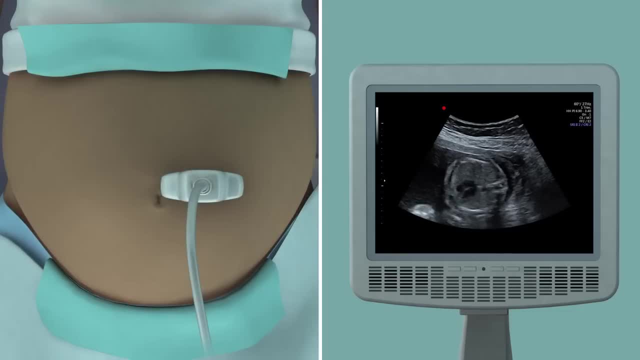 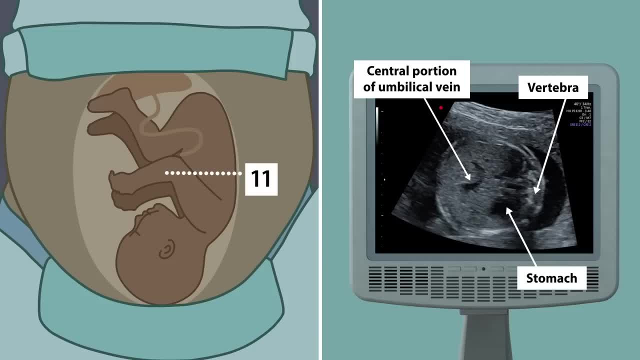 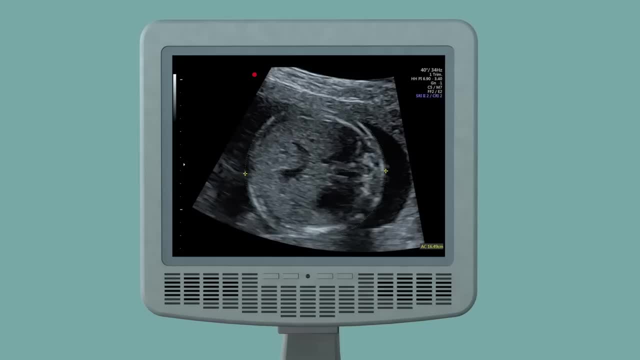 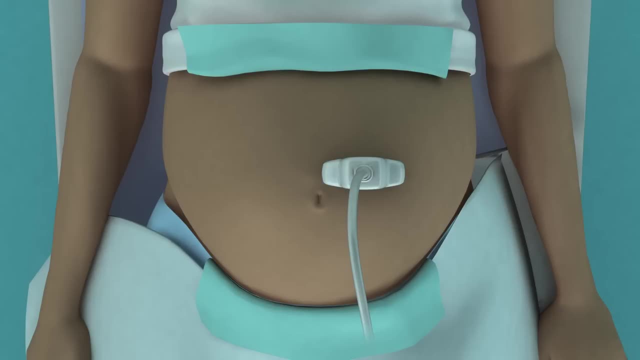 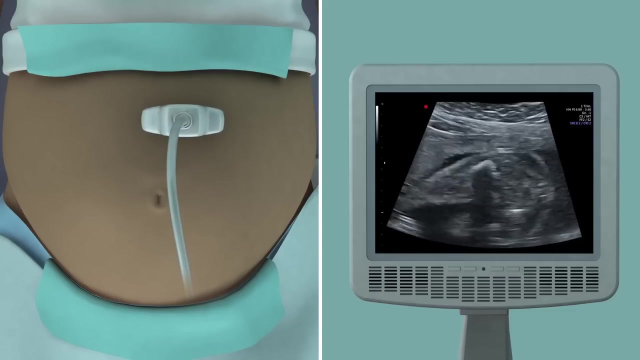 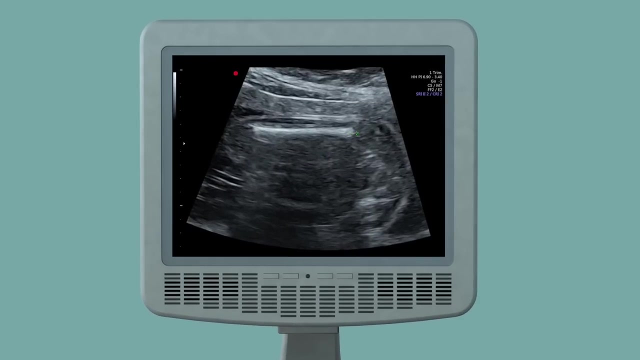 The finally visible are the stomach and a small central portion of the umbilical vein. Best measures for BC measure are the pl weddings. This technique will prevent you from accidentally measuring the humerus. Place the callipers at each end of the femur and measure the longest visible diaphysis. 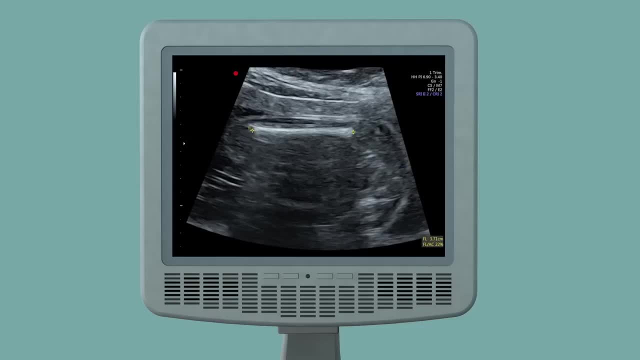 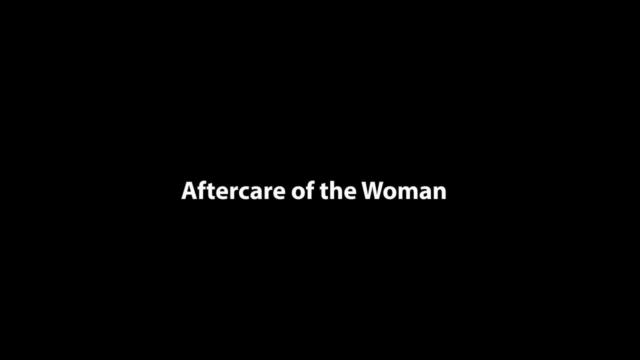 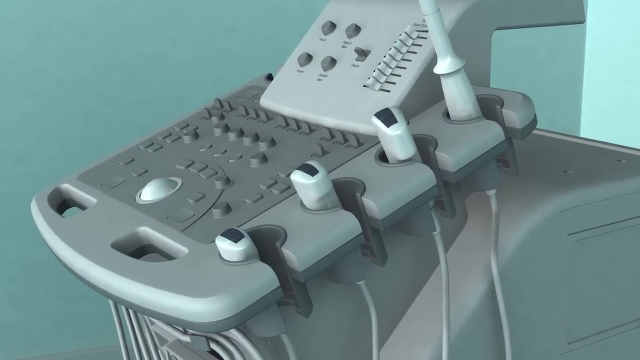 Don't include spur artefacts on the ends of the diaphysis and be sure to measure along the long axis of the bone. The scanning procedure is now complete. Clean the probe and return it safely to the probe holder on the ultrasound scanner. Clean the woman's abdomen and allow her to sit up. 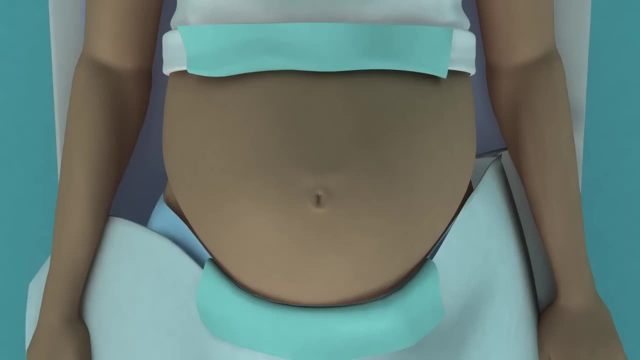 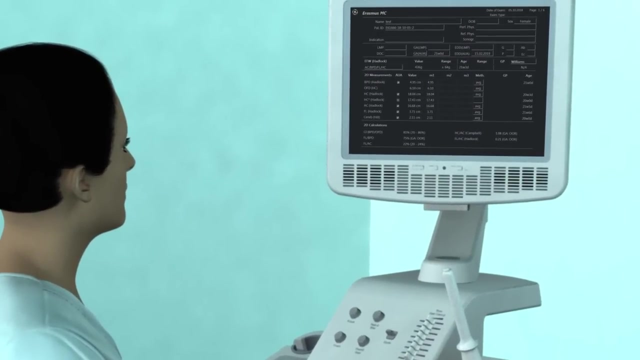 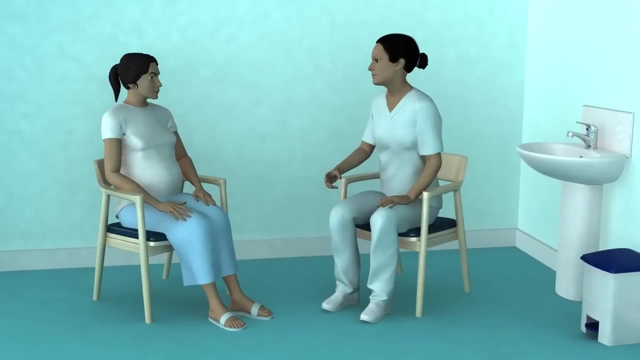 Now wash your hands. Bring up the report mode on the ultrasound screen and check the measurements. Explain the scan results to the woman and give her the opportunity to ask any questions. Provide her with a handwritten or printed report which she can then pass on to her caregiver.